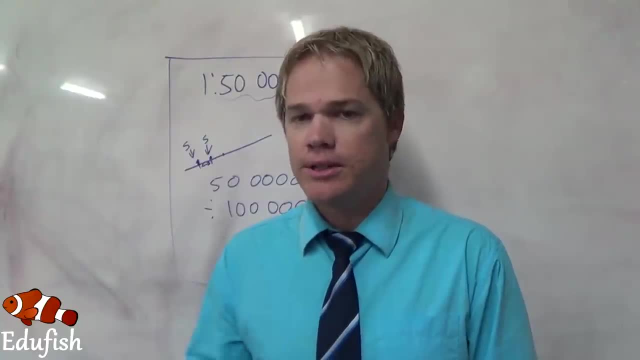 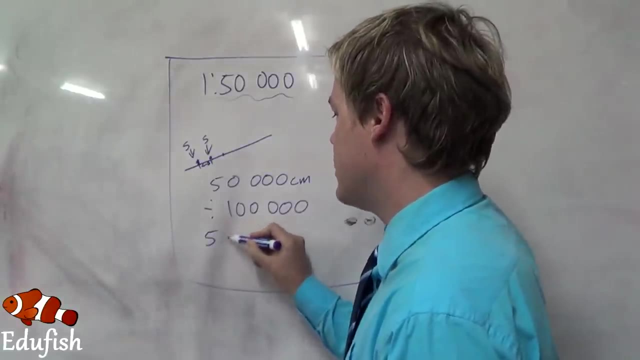 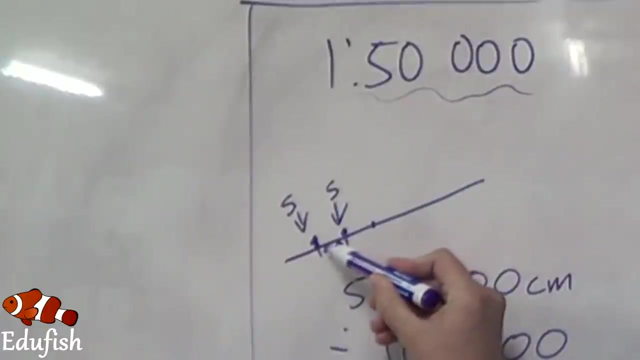 thousand centimeters in one kilometer right now. if we divide 50,000 centimeters by a hundred thousand, then it will give us an answer of 500 meters. so, in other words, this little distance that you see here on your map from from this shop to that shop equals or represents 500 meters in real life. 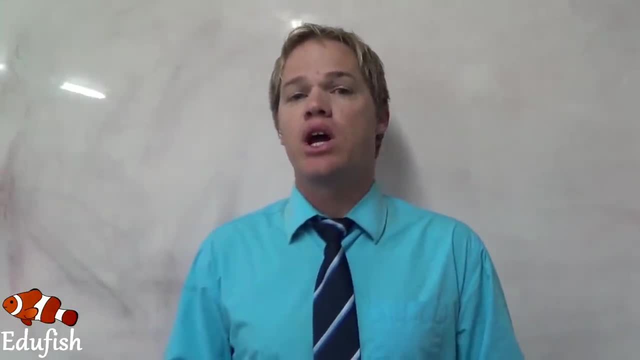 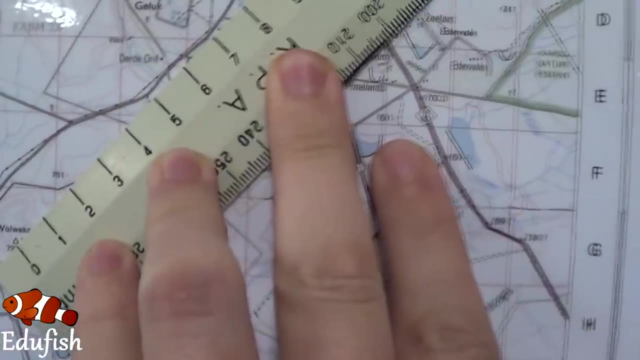 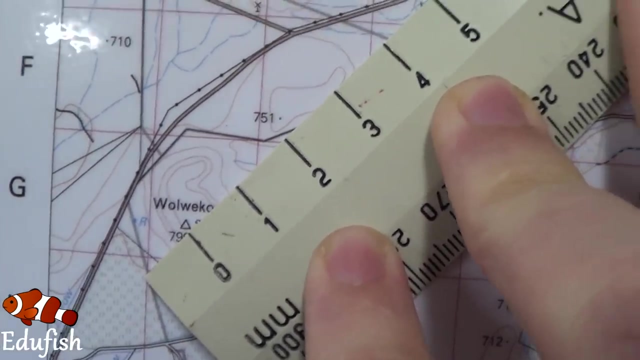 now we are going to look at the map once again and we are going to physically measure the distance between two different places and then calculate the distance. we're going to take it from the highest point um on volvocorp, which is indicated by the triangle there, and then we're going to 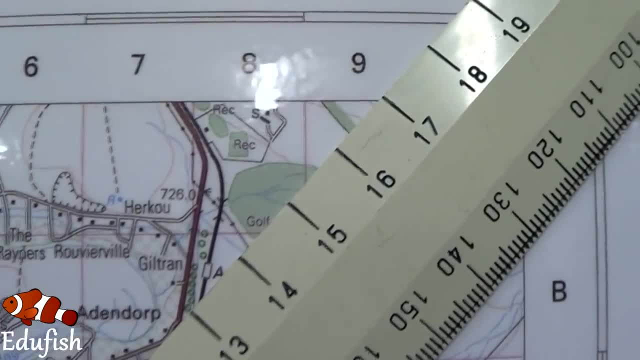 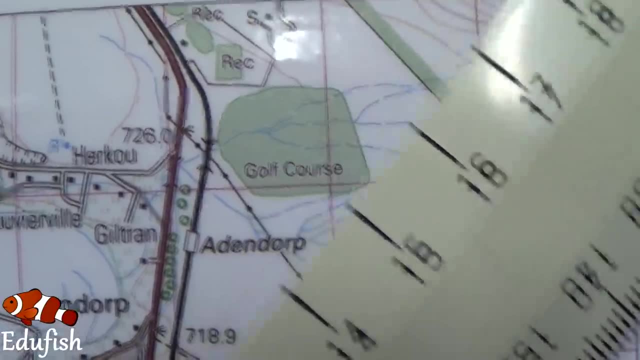 measure all the way to the golf course. we're going to take it to the right, to the middle of the golf course, and we will find that it's more or less exactly 15 centimeters. right now that we've taken the measurement and we know that it's. 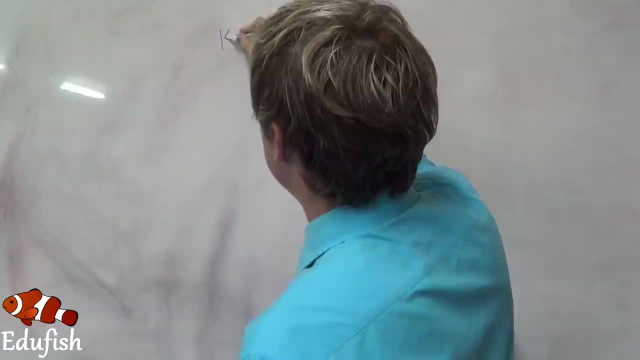 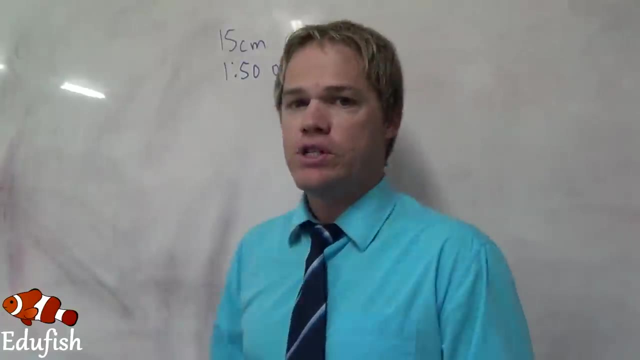 15 centimeters between those two places. we can write it down and we can say 15 centimeters, and we all know that the scale is 1 to 50,000. now, firstly, let's write that method down. the method, the method says distance, distance. 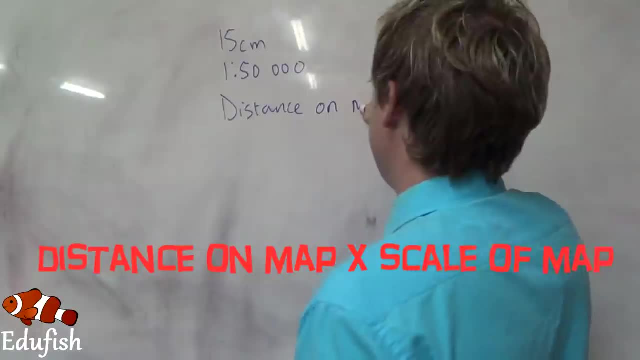 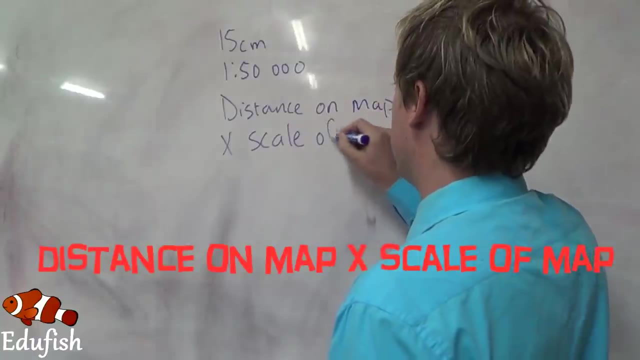 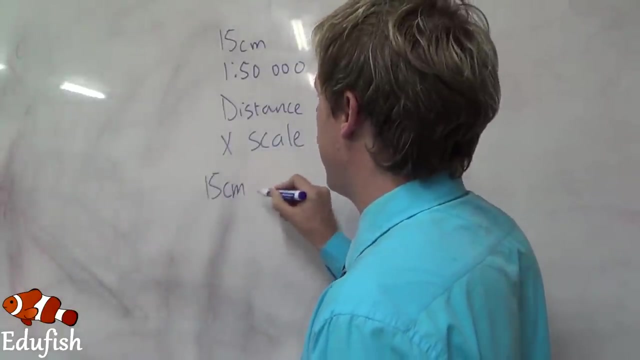 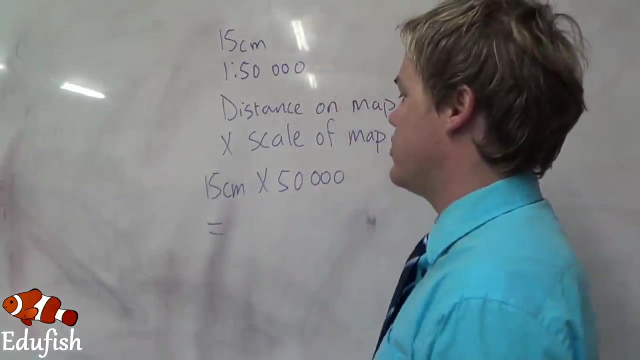 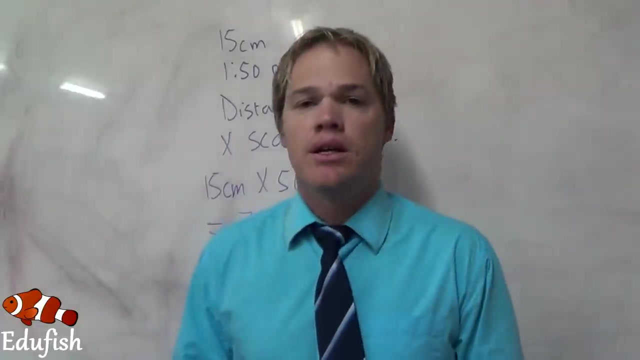 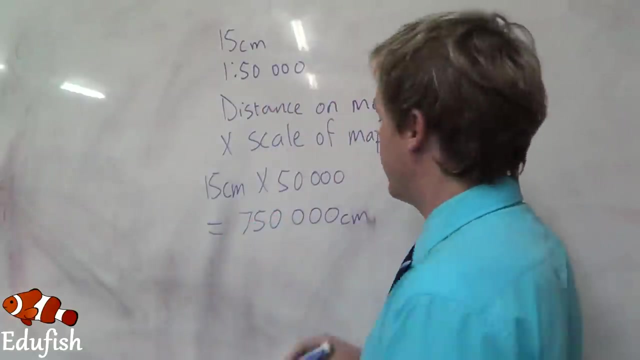 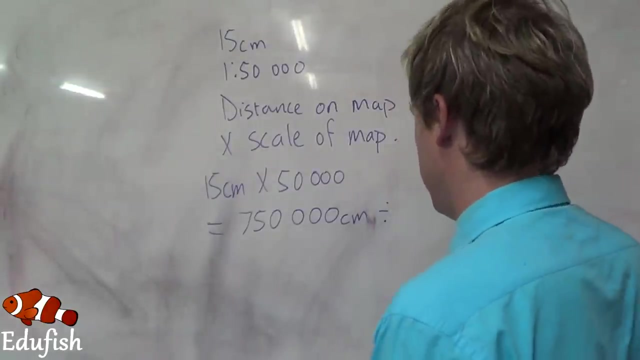 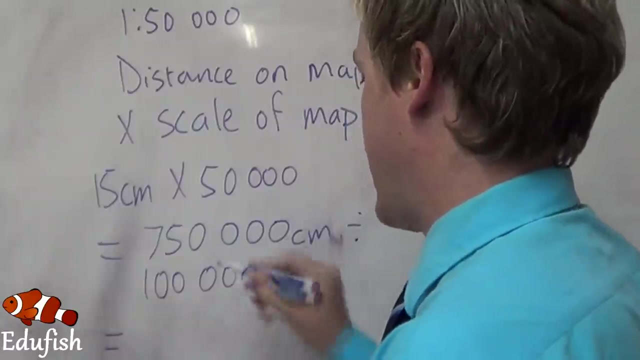 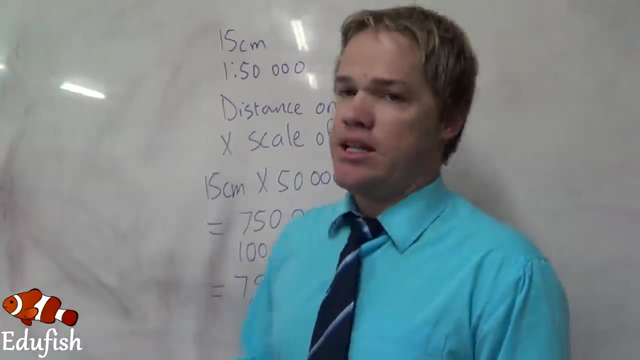 distance on map: times, scale of map. okay, so the distance on the map is 15 centimeters and the scale of the map is 50,000. okay, now, this will give you an answer of 750,000 centimeters. now, like i said, you're never going to say to your friends: listen, i went for a jog yesterday. i ran 750,000 centimeters. now you're going to convert this to kilometers, so you're going to say: divided by a hundred thousand- i'm just going to move it down here, make sure everybody can see divided by a hundred thousand in order to convert it to kilometers, and it will give you an answer of seven comma five kilometers. that is how simple it is, people. now